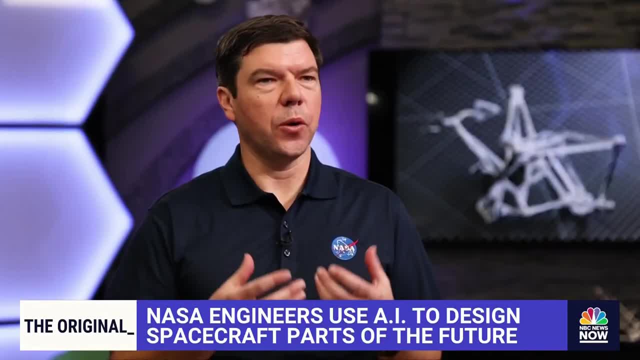 spacecraft together. The first thing is to get the requirements. you know exactly what the part has to be. The first thing is to get the requirements. you know exactly what the part has to be. The process starts with NASA leadership, Tappy McClelland's team to bring two components of a spacecraft. 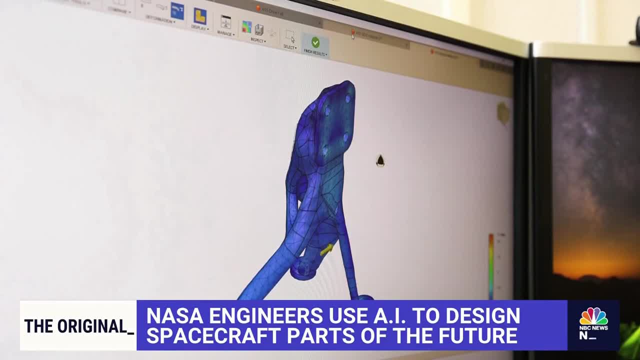 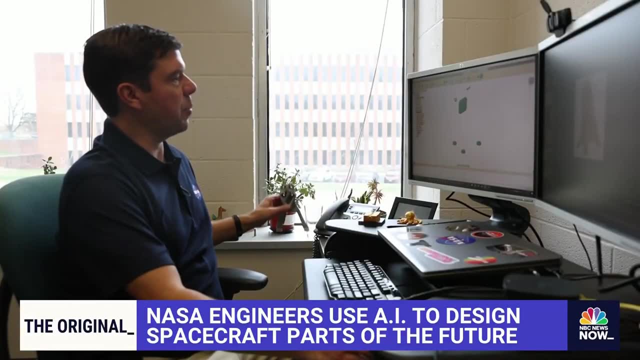 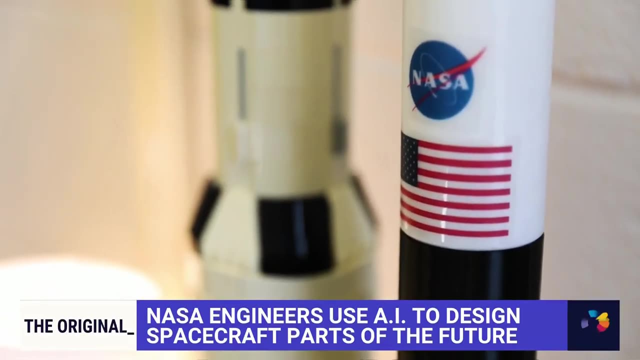 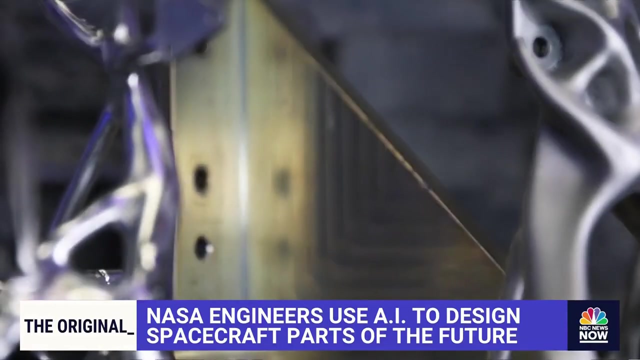 together. The first thing is to get the requirements. you know exactly what the part has to be. M technology allows NASA engineers to shorten the time it takes to develop specialty parts for spacecraft From months down to just days. Plus, the parts are lighter, stronger and they use less material than most human designs. 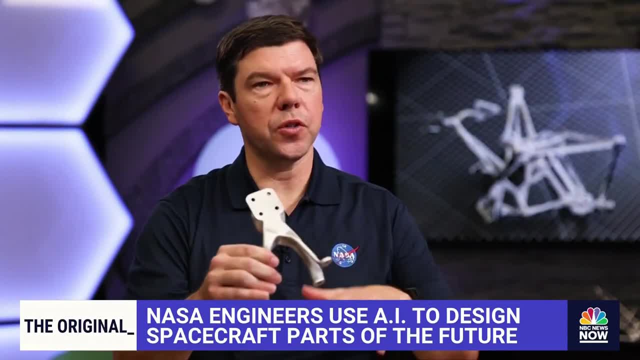 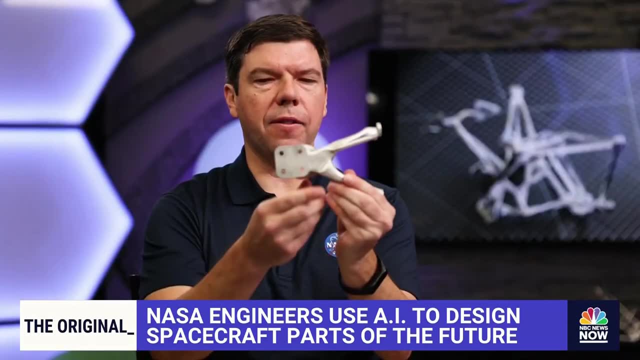 This is a bracket for the excite mission, which is a balloon experiment that goes up above most of Earth's atmosphere and actually looks at exoplanet atmospheres. So this is just sort of a simple bracket that holds an optical assembly to the back of a telescope. 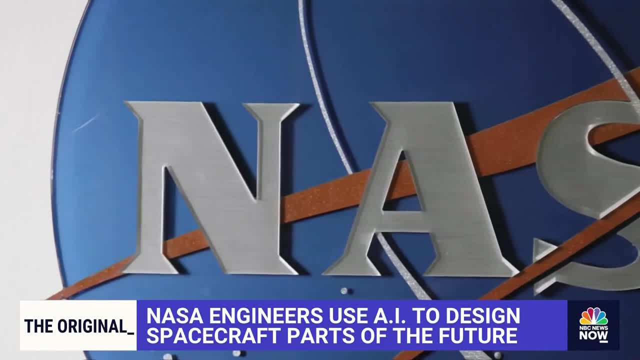 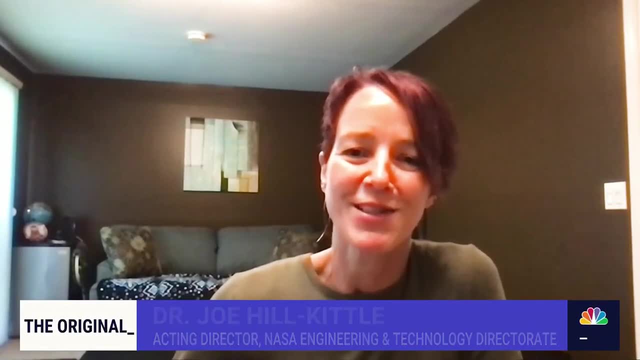 Dr Jo Hill-Kettle leads NASA's Engineering and Technology Directorate. The most important thing to me is this is the future of NASA and the future of spaceflight and the future of space instrumentation. She says the technology could be a vital resource for future missions. 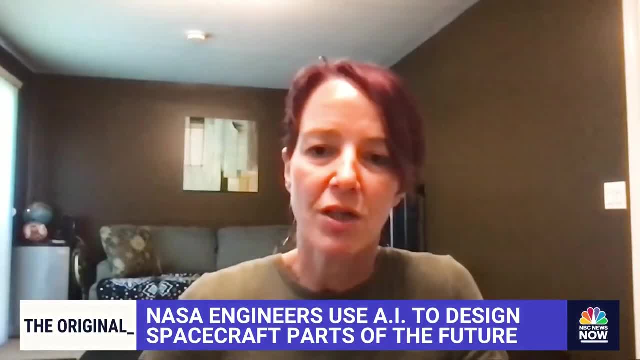 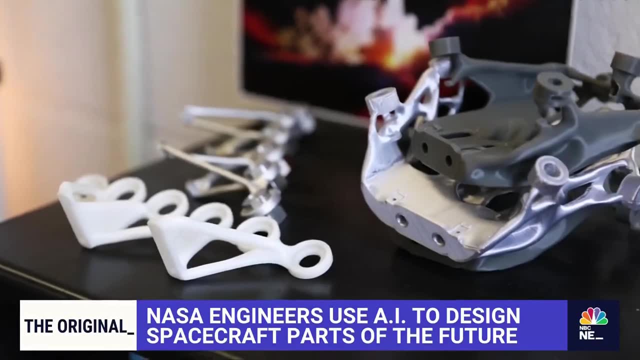 If we're going to have a sustained presence on the lunar surface or eventually on the Mars surface. the additive machine creation of these parts and the rapid turnaround would allow those folks to be able to perhaps fix things in real time, be able to build things off-planet. 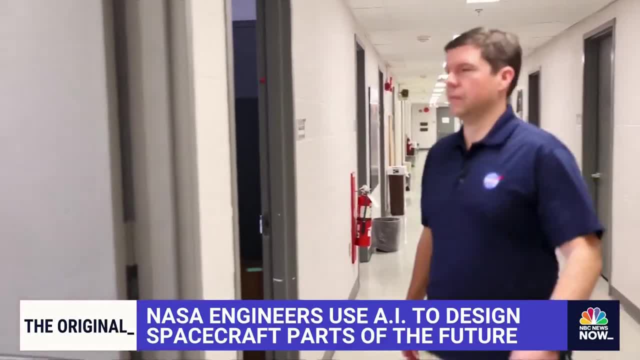 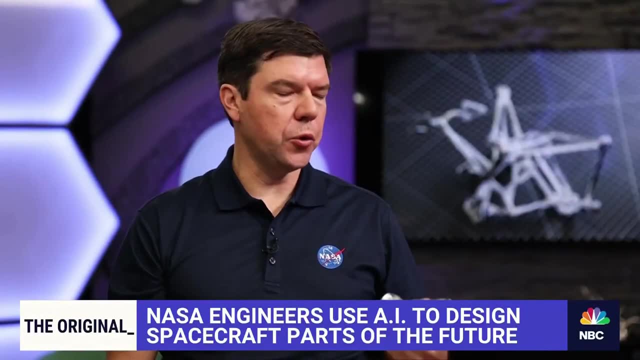 But McClellan says aspiring engineers shouldn't worry. This technology will not completely replace humans, at least not yet. Where it stands right now and where I see it in the near future is that it's kind of like a consultant that allows us to be more productive. 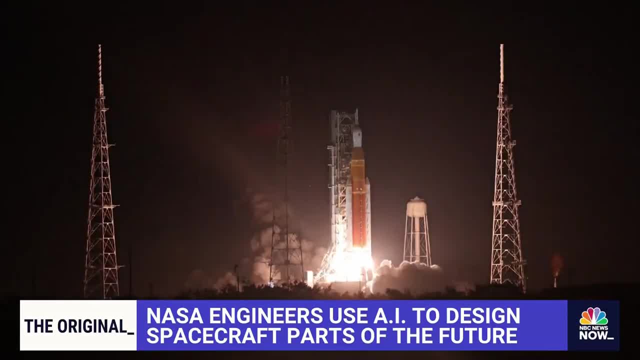 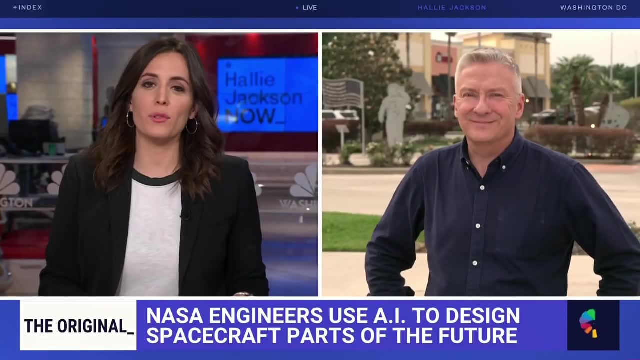 but the human designers still need it. Artificial intelligence: improving spaceflight one piece at a time. Tom Costello is joining us now, live from Houston where he's been covering the latest on the Artemis mission. So let's get back to that: Artemis 2 and this announcement today. 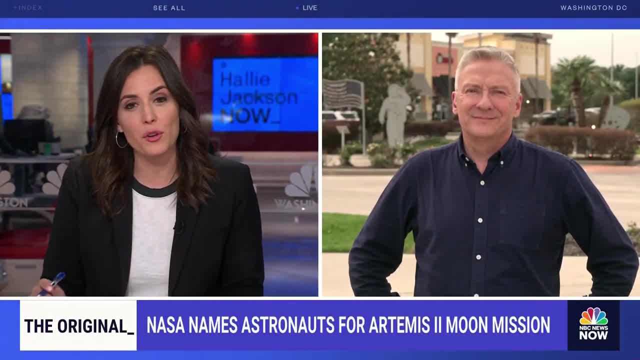 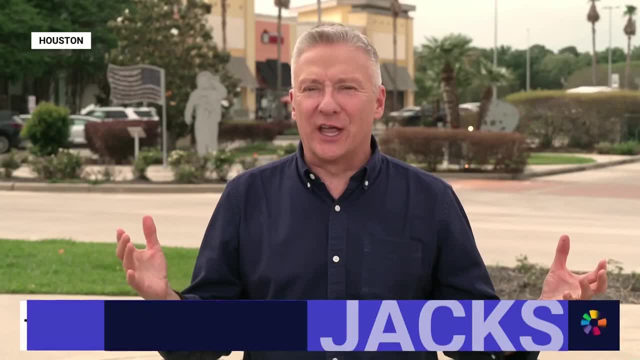 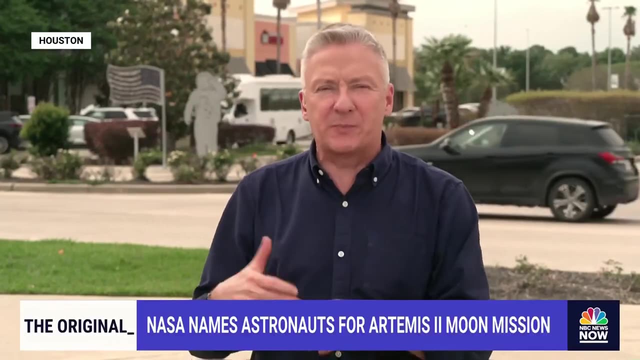 Talk through, kind of this new generation of astronauts, what they're saying about the future here. Well, they're thrilled, as you could imagine, And this entire aircraft hangar today was filled with people who are absolutely amazed, Absolutely thrilled. Other astronauts, astronauts' families, NASA staffers, politicians.